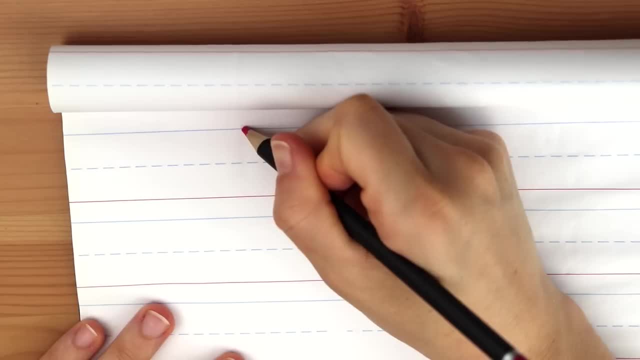 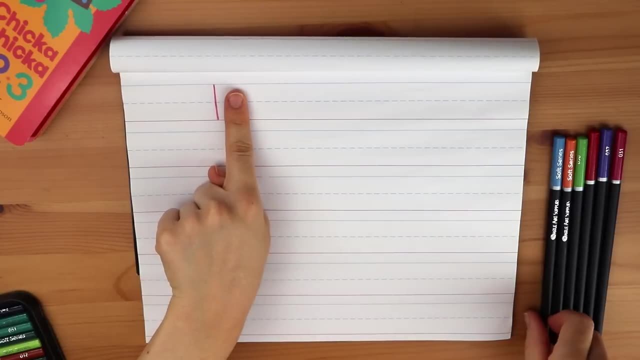 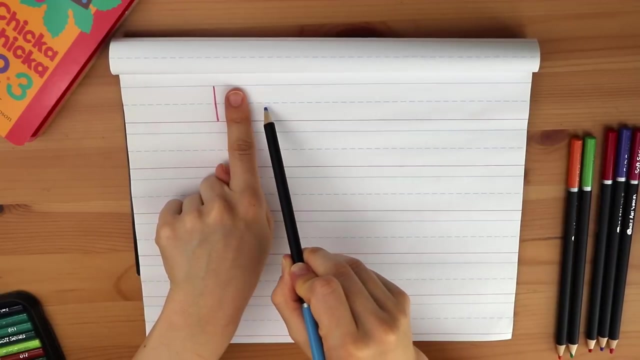 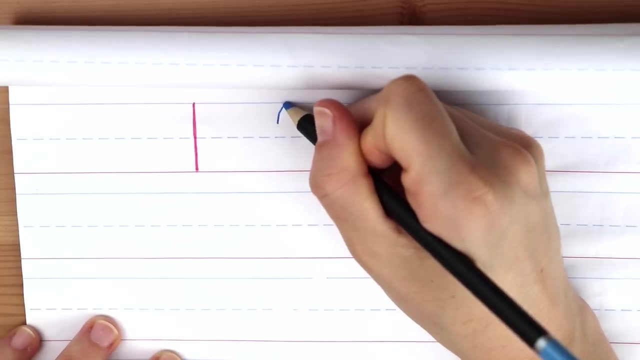 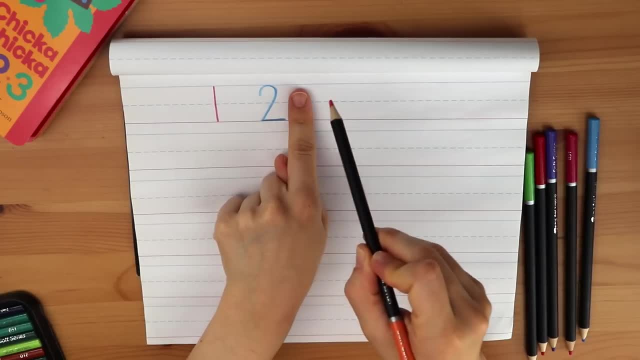 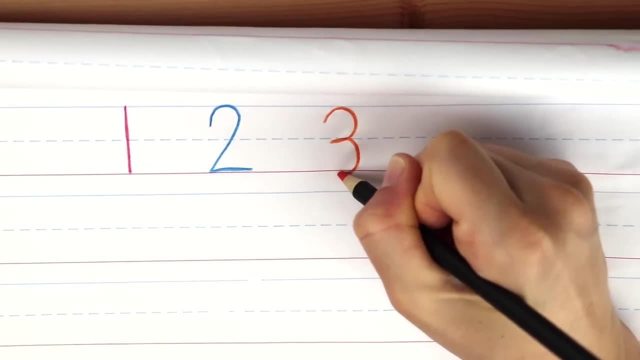 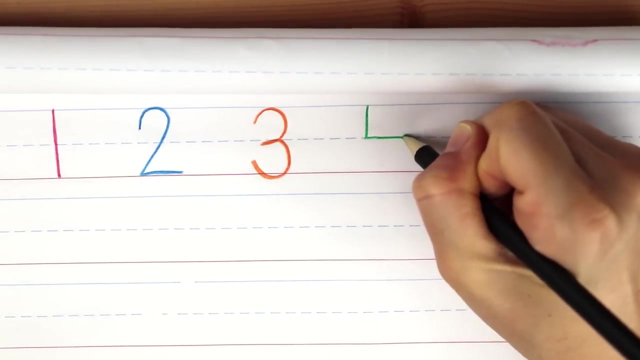 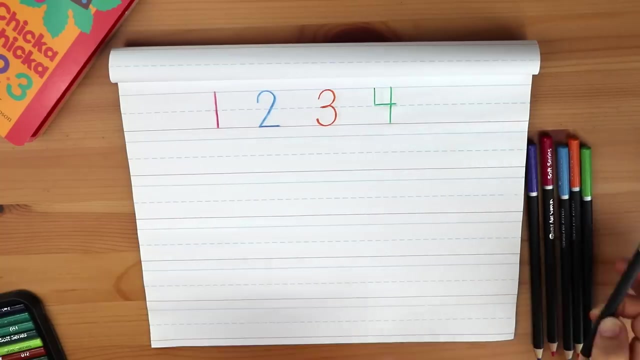 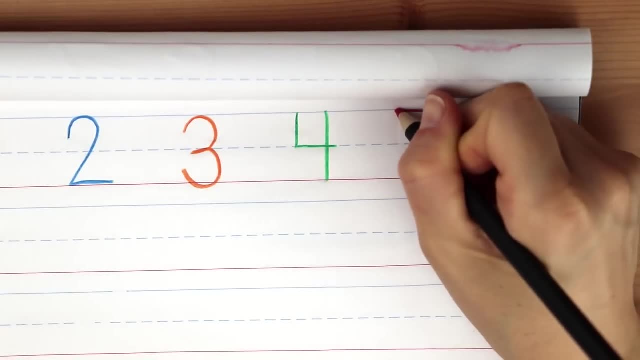 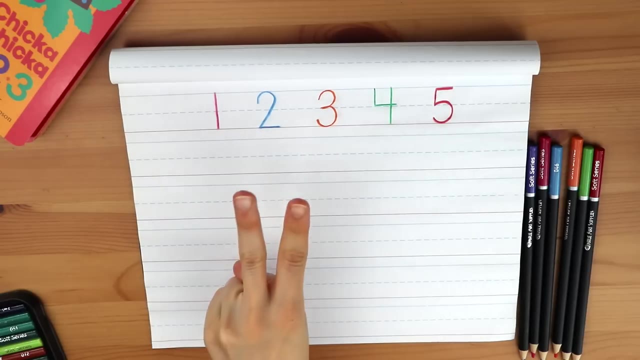 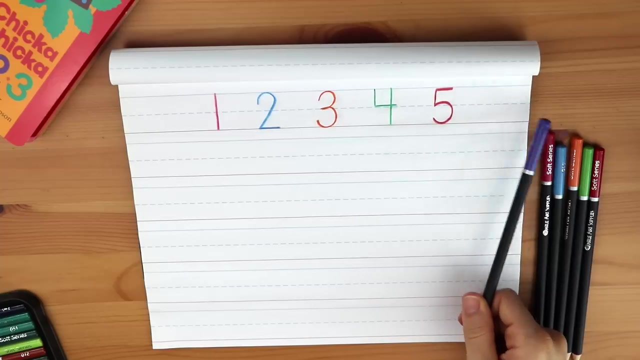 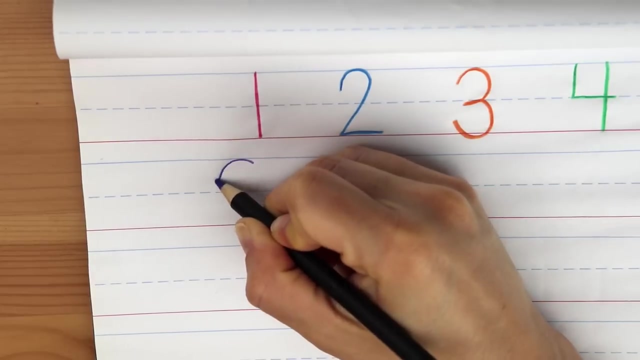 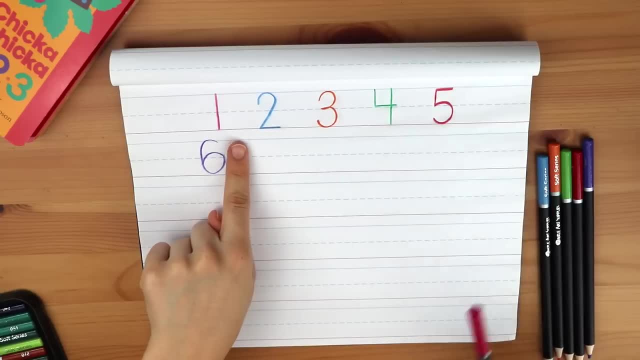 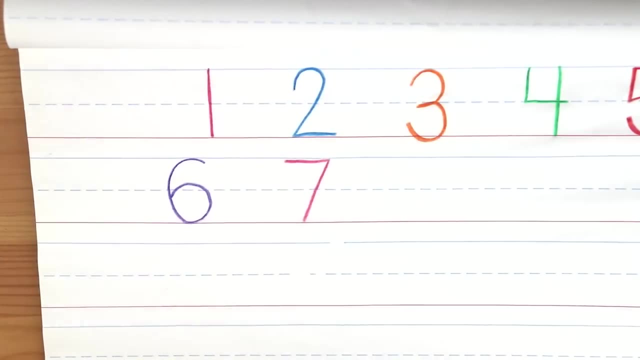 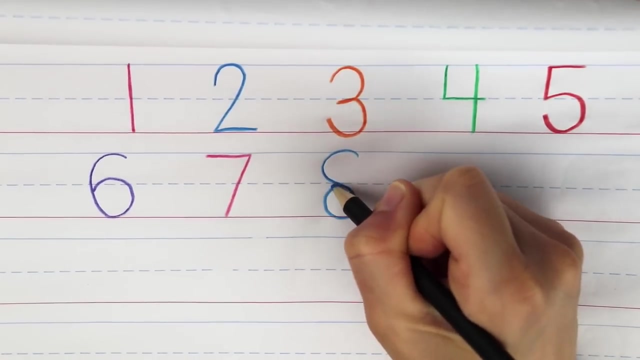 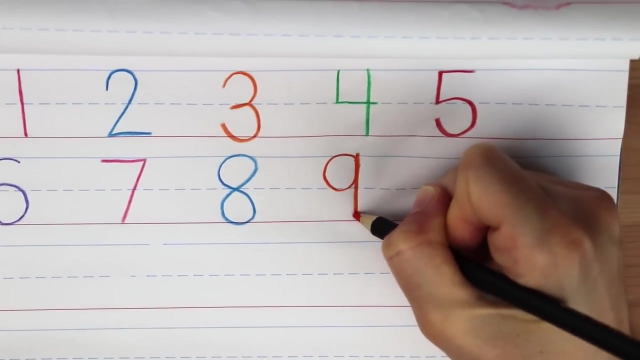 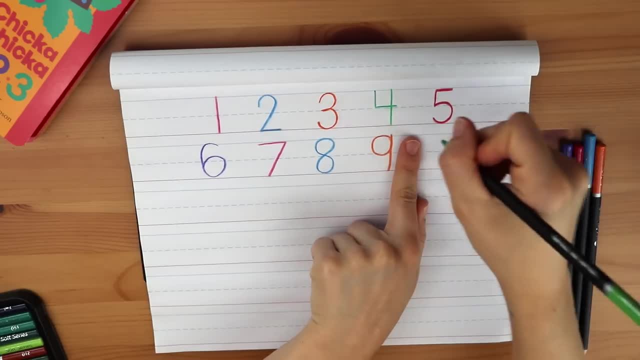 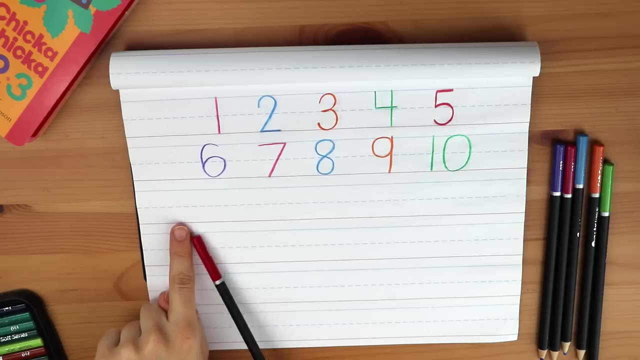 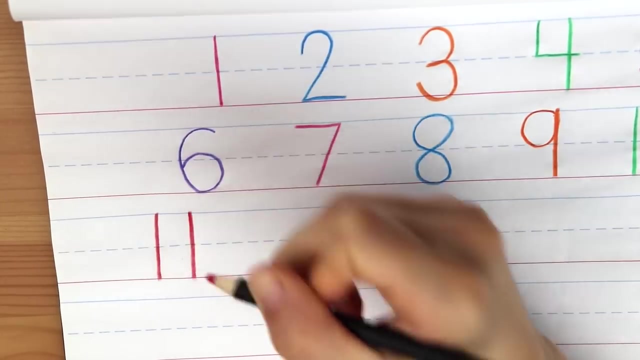 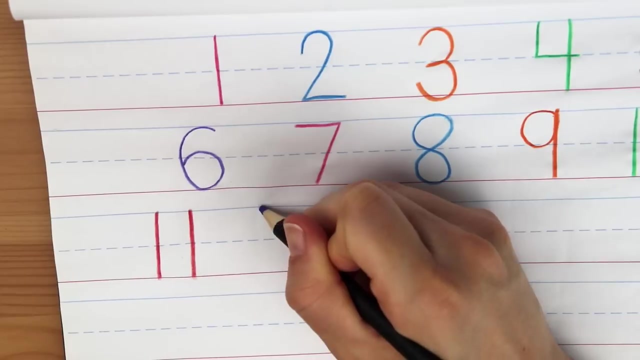 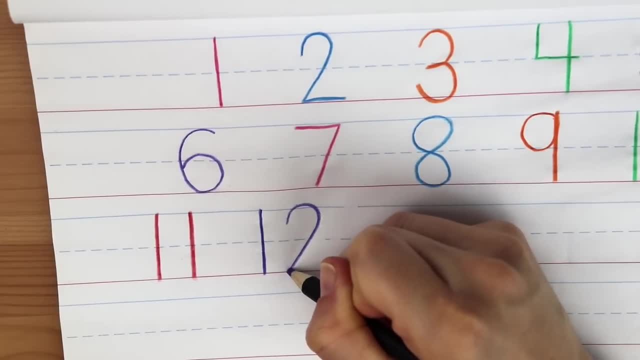 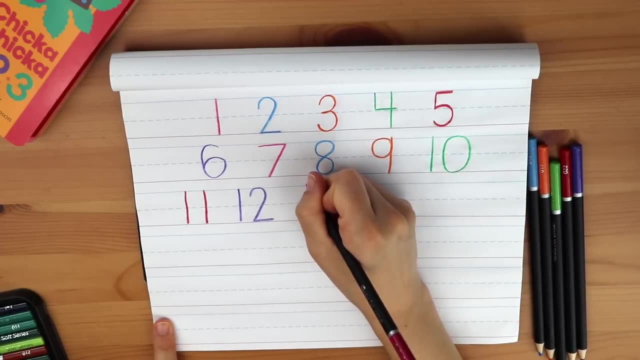 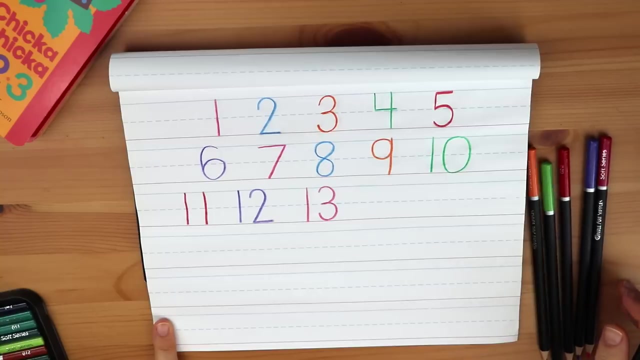 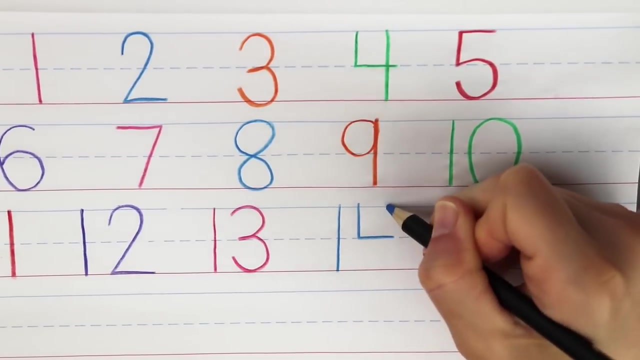 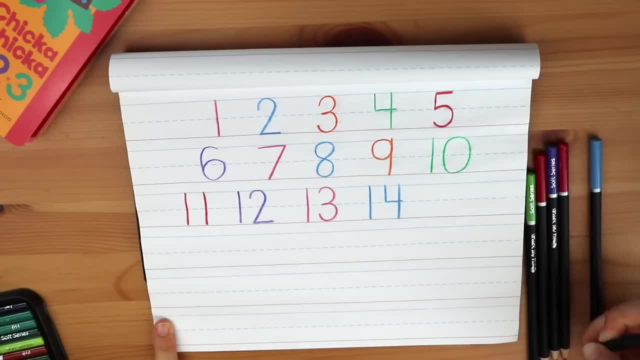 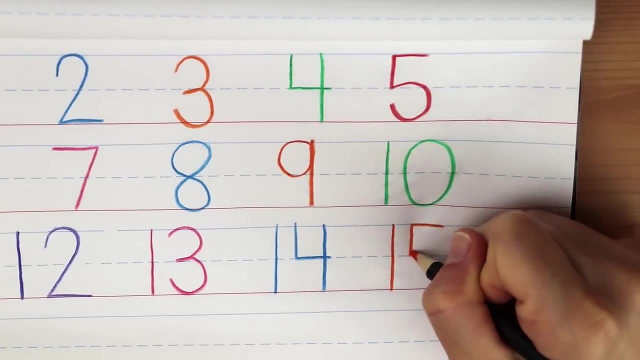 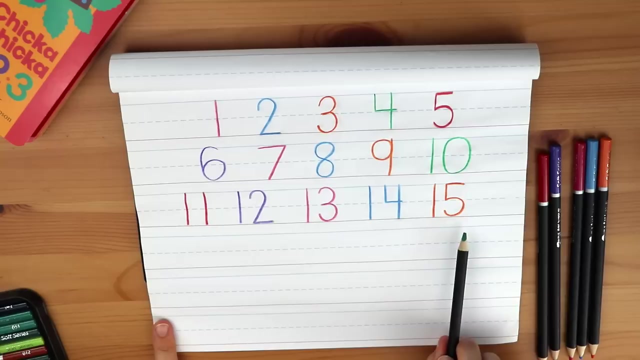 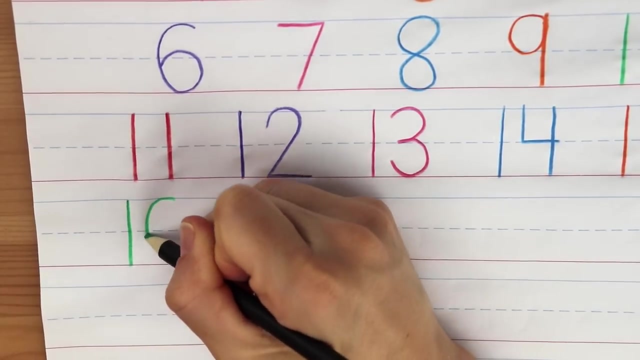 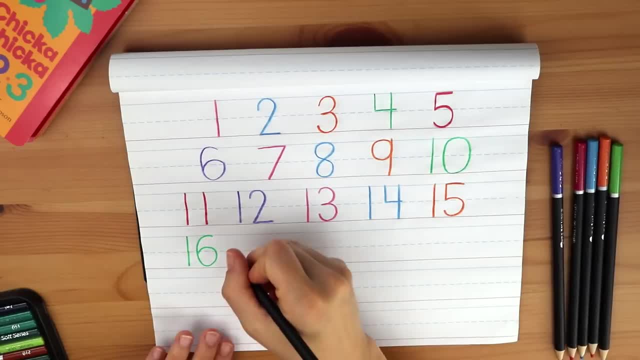 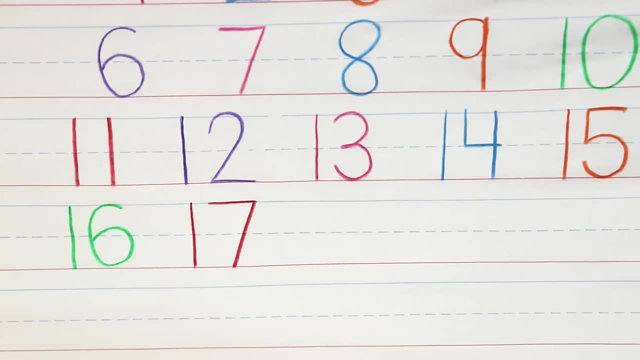 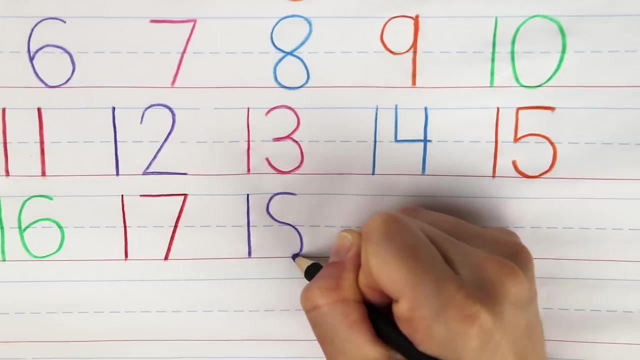 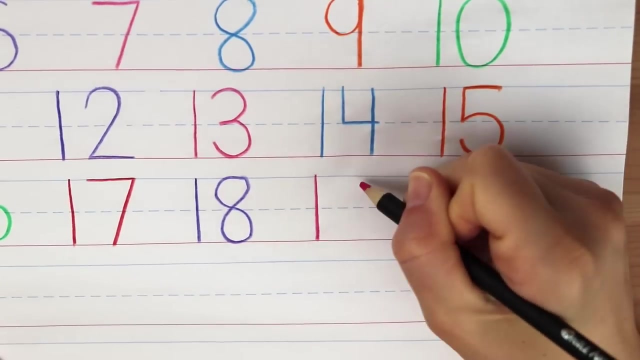 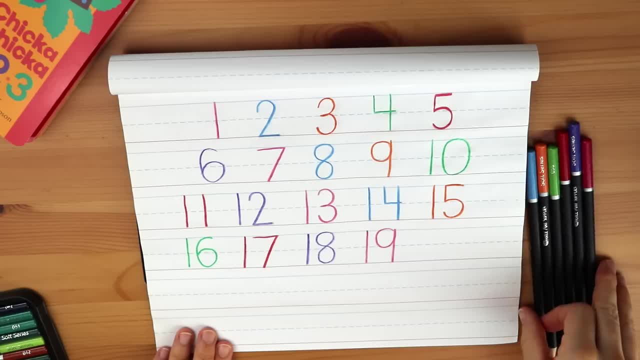 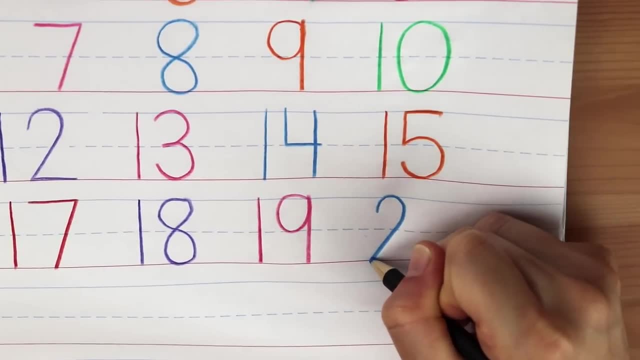 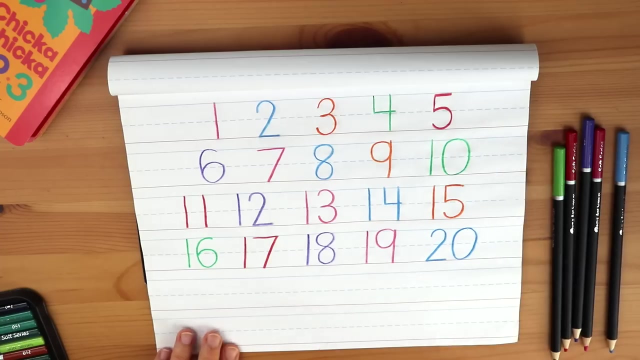 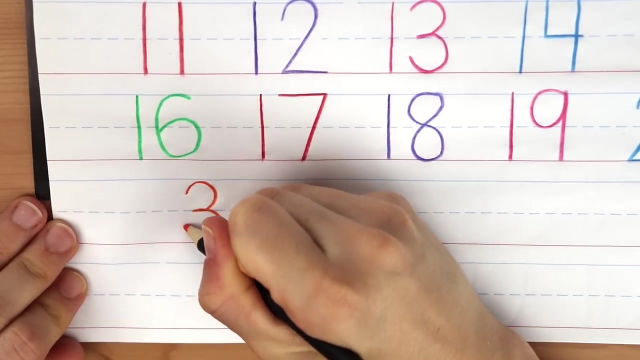 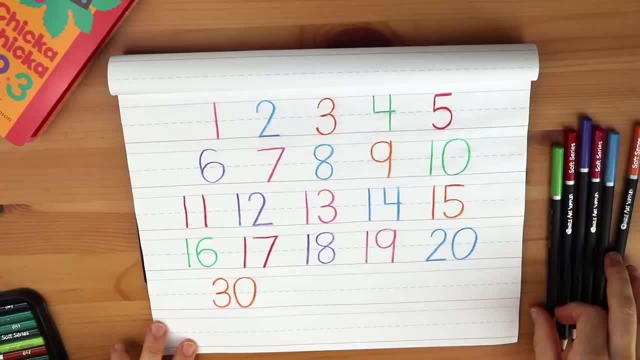 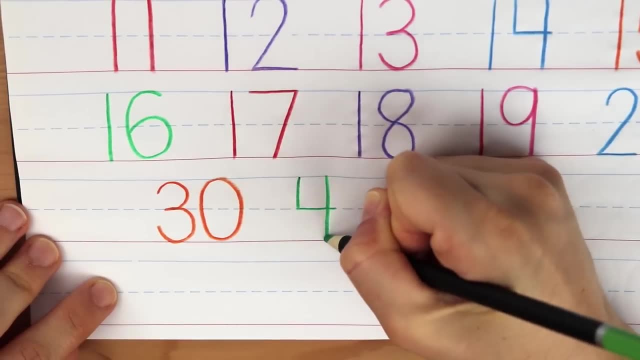 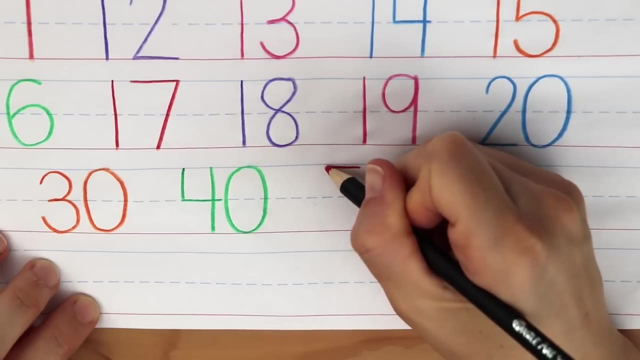 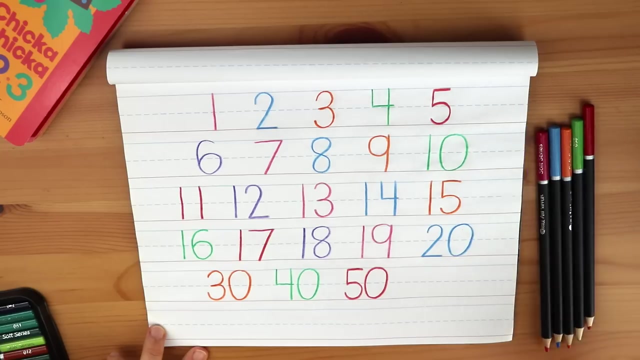 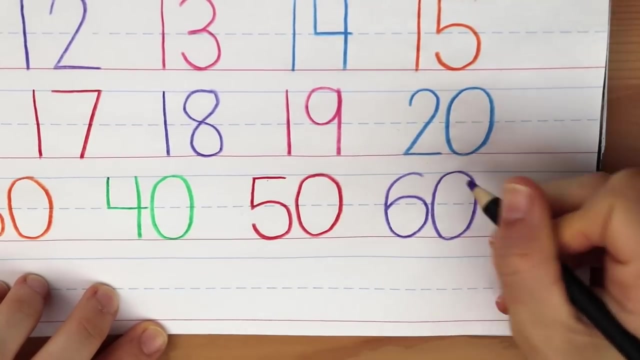 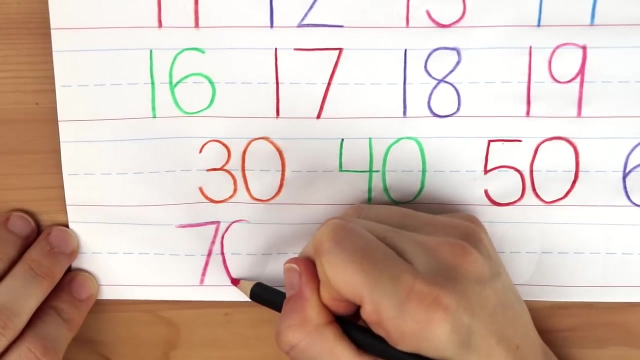 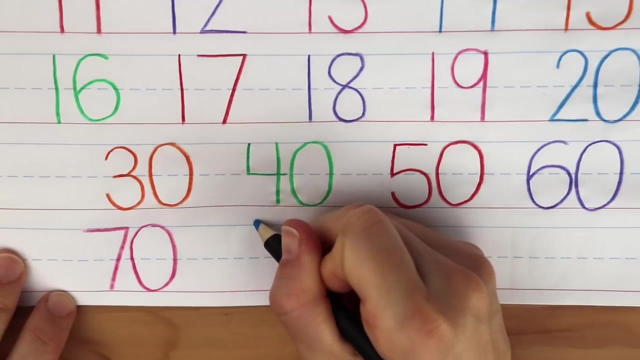 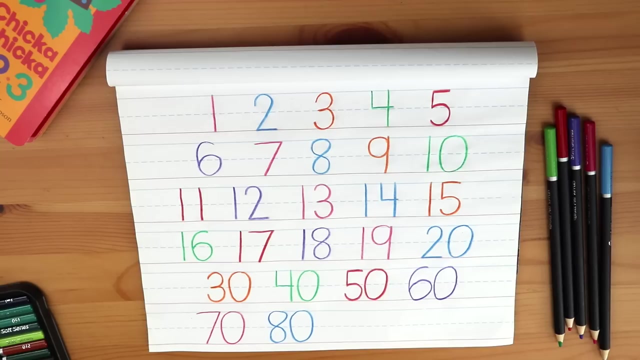 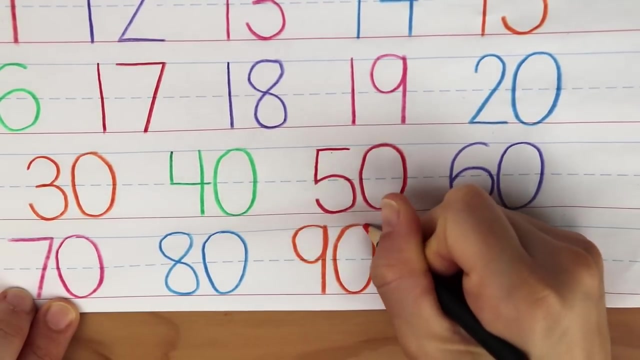 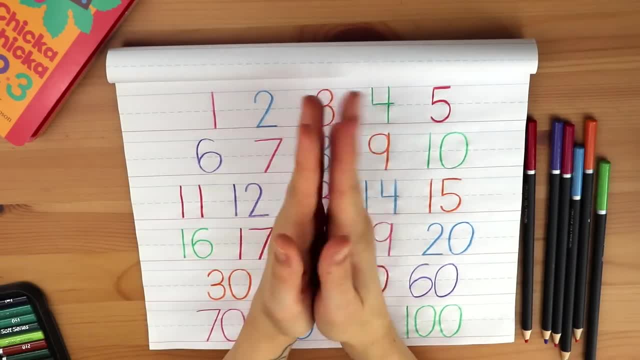 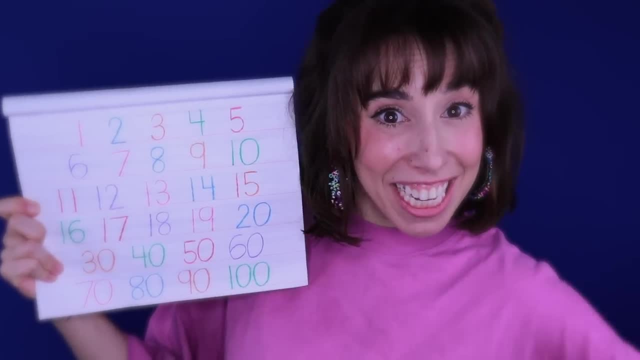 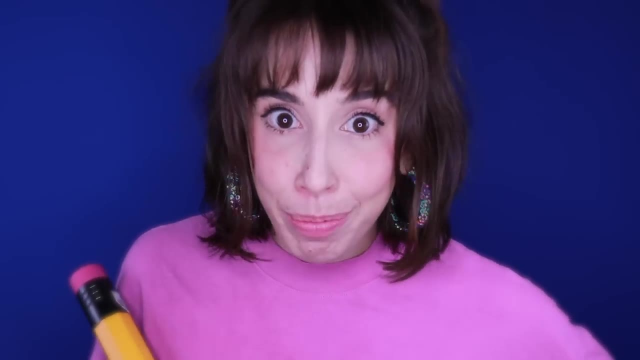 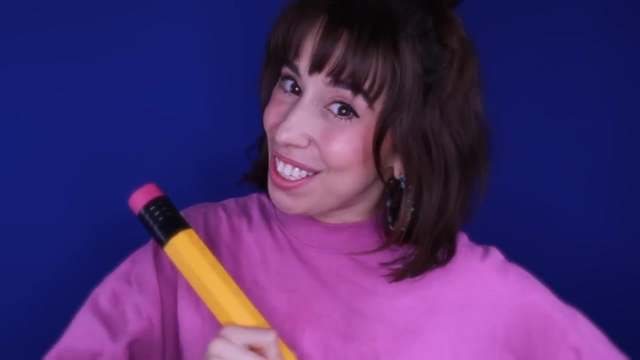 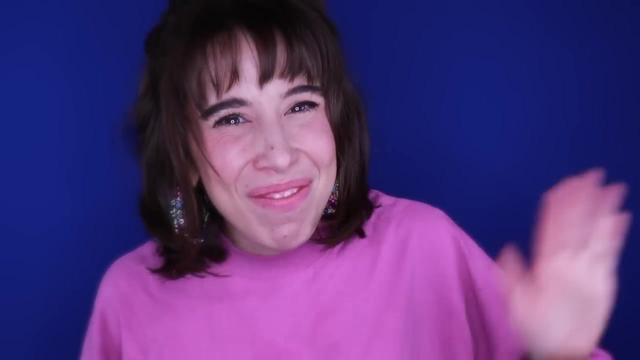 Hooray, You did it. Thank you for writing with me today. Now you can practice writing and counting up to one hundred or even more. Please subscribe to my channel for more books and more fun. See you next time. Bye-bye.